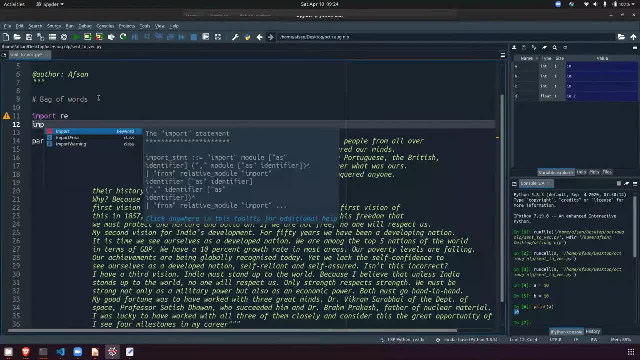 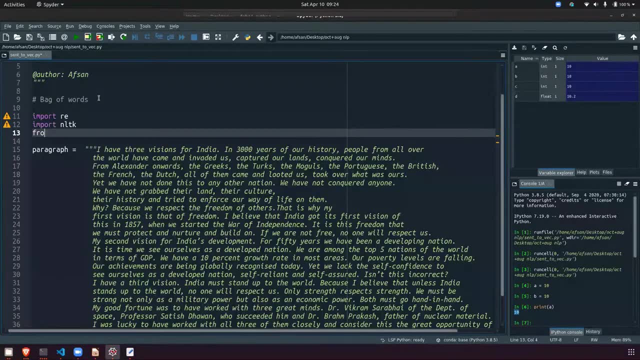 Regex, Regex, Okay, So import, And then tk, Then we have to import. So basically we will import all the libraries, all the packages which are essential for pre-processing. Okay, Data cleaning, Or data Data cleaning as you call, it, is in NLP, So from nltkcorpus. So basically the very 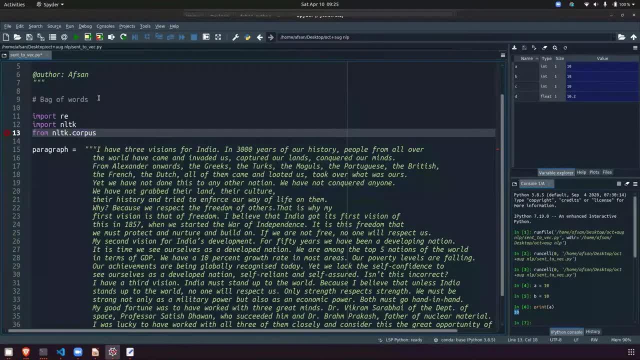 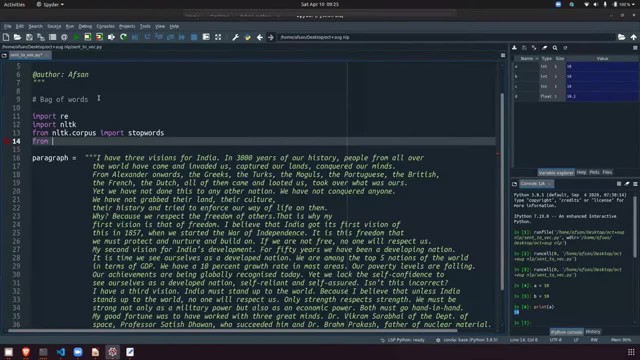 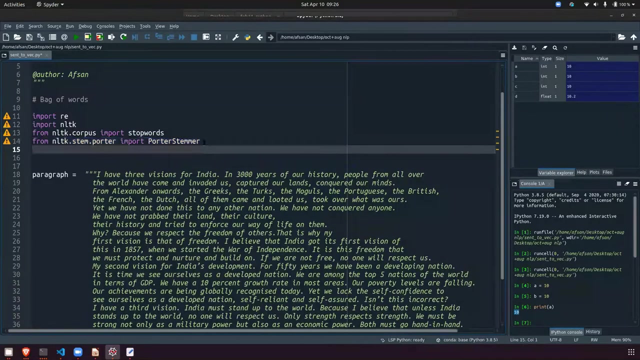 work with any one of these. so we import both for now. okay, so nltk dot stem dot porter import. so nltk dot stem dot quota import for the schema supporter. uh, and the same thing. so limitizer, if you remember there's something called as word net limitizer in nltk, so you can. 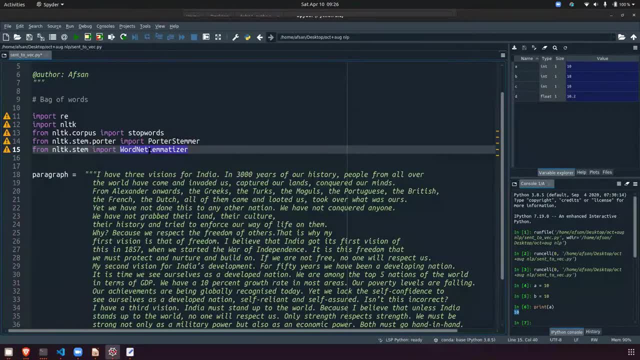 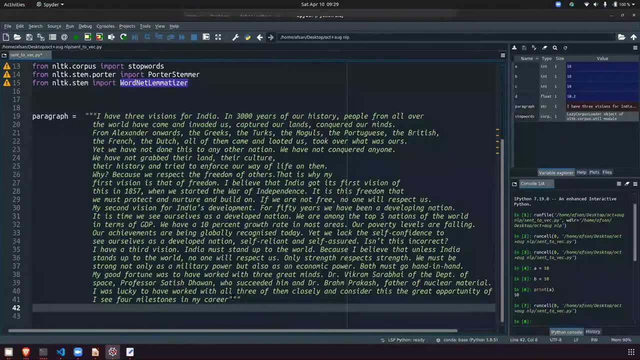 use any other libraries. okay, so i am using nltk just for demonstration. you can use pc, you cannot any libraries, okay, okay. so these are the important libraries that we work with now. how to now in a jupyter notebook, step by step, i have shown with the example that, how you do. 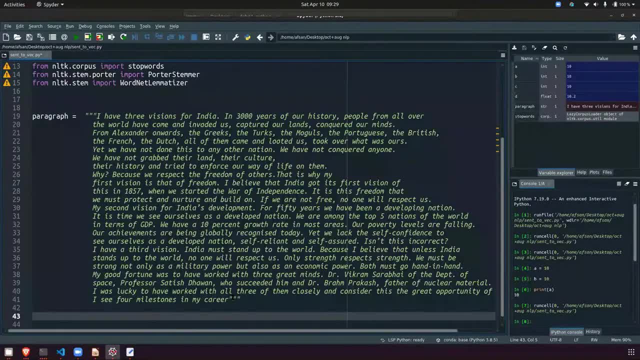 how you remove stoppers and how you convert to lower, then split, then convert. this is this we have done without using, with the help of a small example and with the help with a in one, one shell. okay, now, how to code for a particular use case. so what we have to do is we have to write a follow. 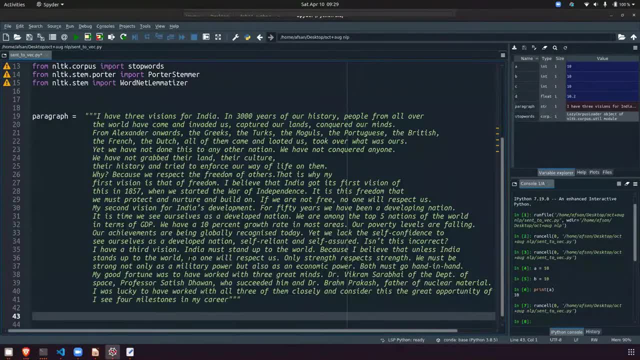 now. okay, so we have to write a follow thing. what you have to do is: so: can you tell me what is the first thing that we have to do for text speech processing? what is the first thing? okay, so converting to lowercase or uppercase, and then next tokenizer- tokenization. exactly okay, so what i will do is uh. 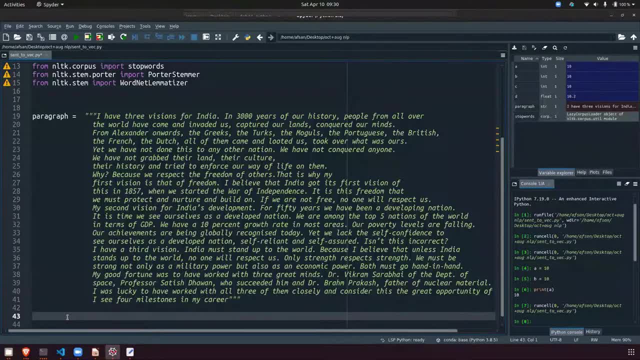 so how to how to? so i will here. i will use tokenizer. okay, so how do you send this tokenizer in nltk, any idea? and then tk dot, then underscore tokenize, so send underscore tokenize and then bracket paragraphs. okay so, paragraph paragraph dot. okay so. okay. so, if i run this now so you can see on the left hand side, everything is getting stored so. 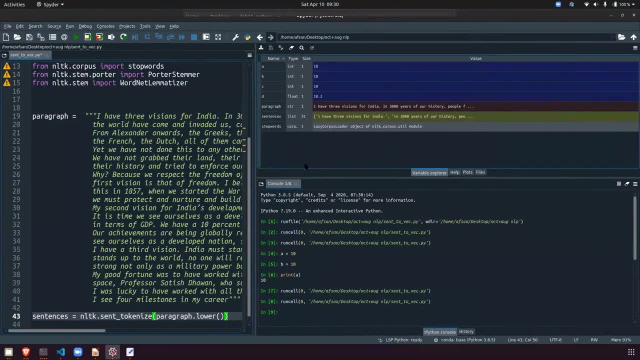 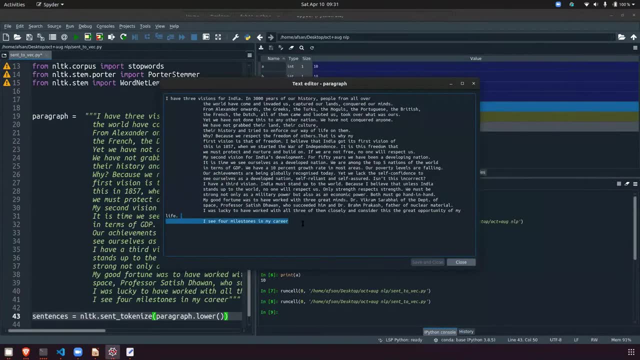 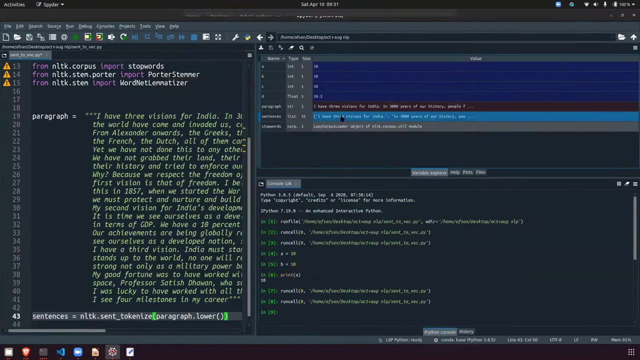 you can see literally that, whether the sentence is converted or not into a lower case, okay, so this is a paragraph. so if you double click on that, a new window will get open. so you can see: okay, this is your text, this is your text and this is the original paragraph variable and the sentence. 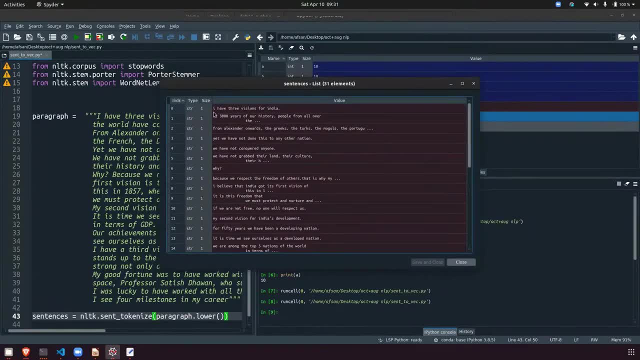 variable if you double click on that, so you can just compare the two and you can see. okay, everything is converted into sentence organizer. basically it's a list of value now. so this is the first sentence, this is second sentence, this third sentence, four, five, six and so on and everything. 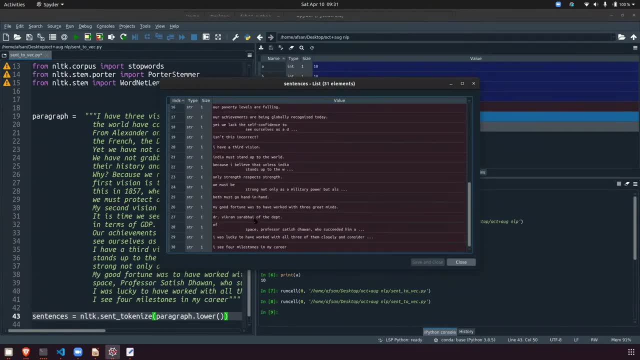 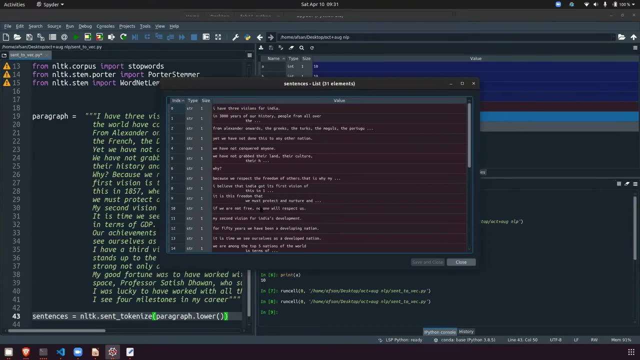 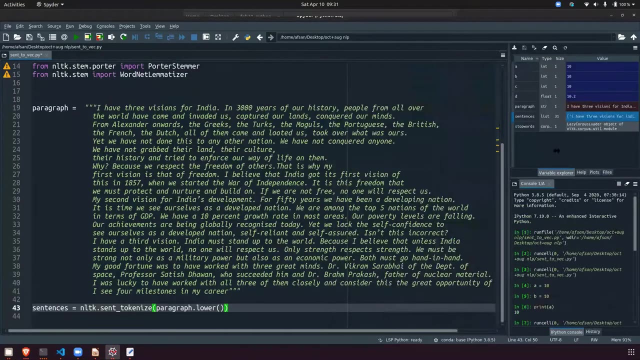 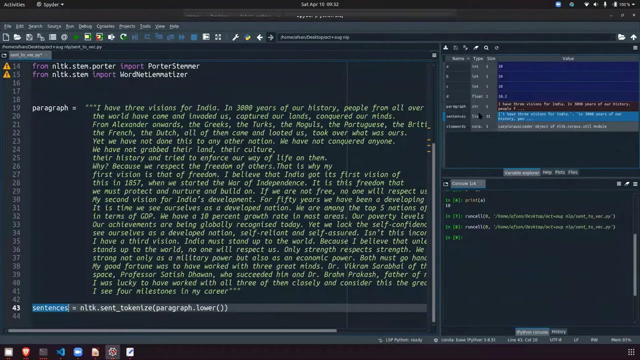 is converted into lowercase. okay. so that's why i choose simple notebook, because visualization is very easy. sorry, no, jupiter's paranoid spider ID. so you saw what is the length of the string. what is the length of the string, what is the length of sentences? okay, so we have seen that, how to convert a lowercase. now the question is so what I want. 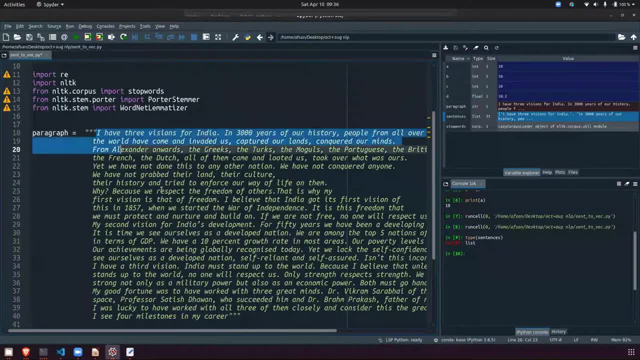 is that I want this particular sentence, okay, this particular sentence, I want to clean this particular sentence. so, basically, you have to remove the stop words. okay, we have to. after remove the stop words, then just lemmatize this, just lemmatize this and then again join. 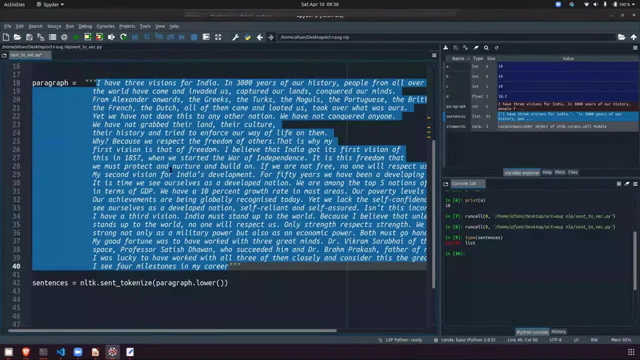 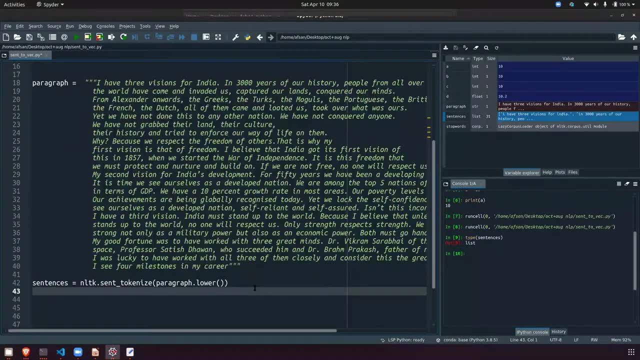 the sentence and I want the same sentence, but the lemmatization should be there and the stop words should be there. okay, so that's the query form. so my query is clear to everyone: that what, what is the next procedure that we have to do now? our image: to clean the data. 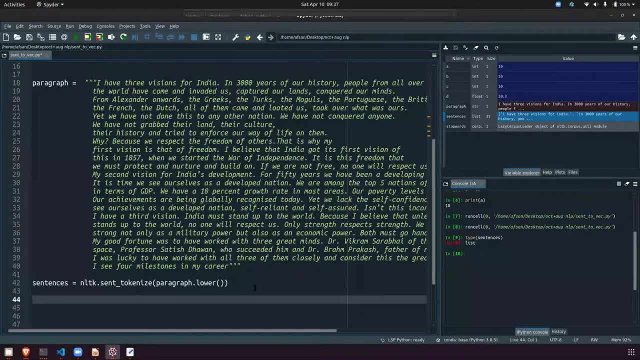 so our image, to clean the data, so lowercase we have done. now we have to split this or we have to word tokenize or anything you can do of your choice, and we have to remove the stop words and we have to stem or lemmatize- basically it's up to you. what if we want to? 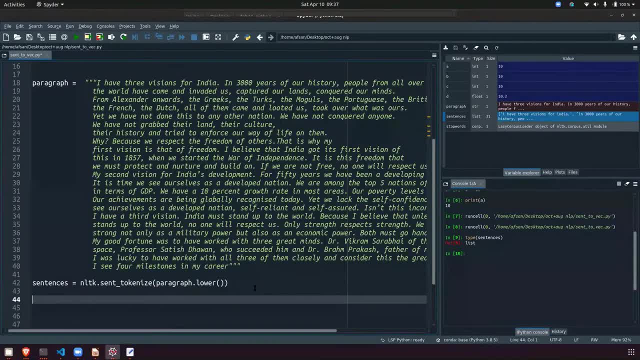 lemmatize or stem, stem, stemize the word. okay, so it's up to you, but you got the point what you have to do. the next: we have to clean the data, okay, so, cleaning the data, so you can apply any method. okay, now what I will do is I will file code, I will code. 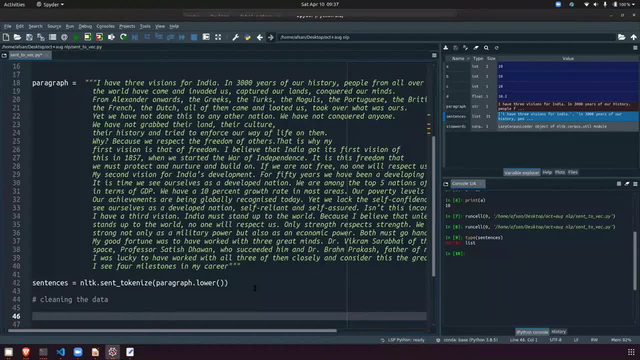 parallelly, you can also code in your own way, but at the end you should get the answer. okay, at the end you should get the answer. so, basically, you should get a single string. you should get a single string where all the words are concatenated means all the sentence you have. 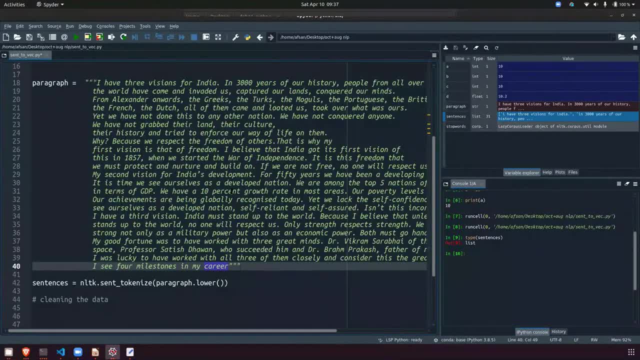 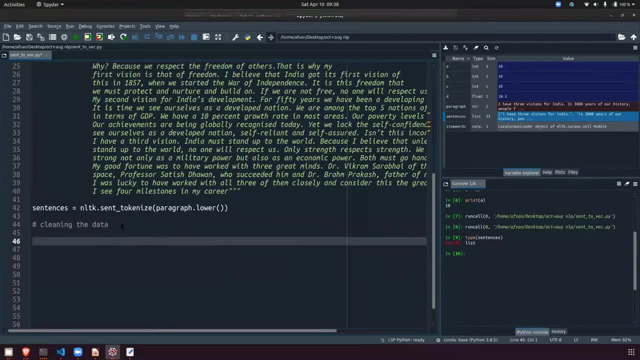 proper sentence with the removal of stop words and the words should be lemmatized. okay, so this is what I will type and it's up to you. okay, so what I will do is I will create a dictionary, I will create a list, so corpus and for I in range. so basically I am running. 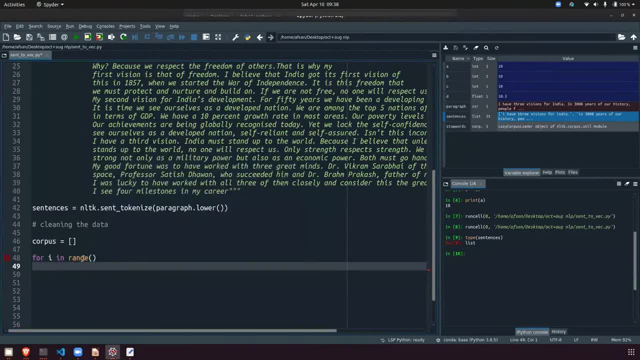 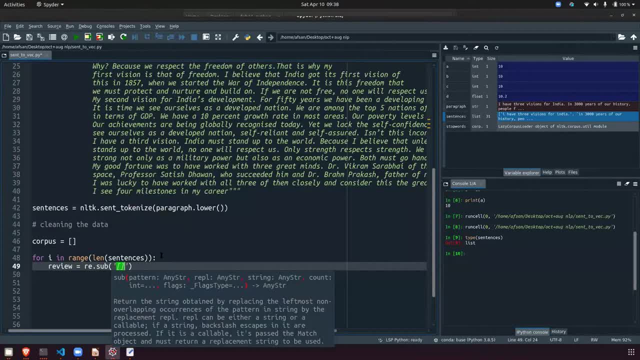 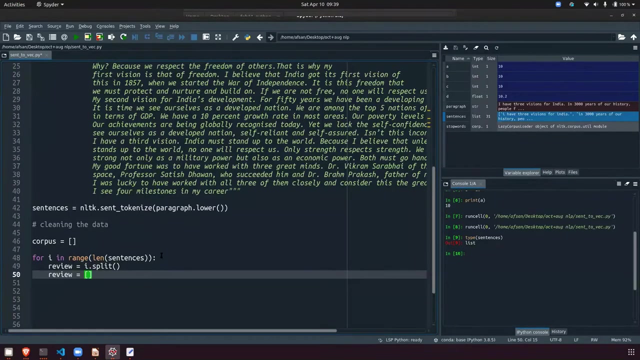 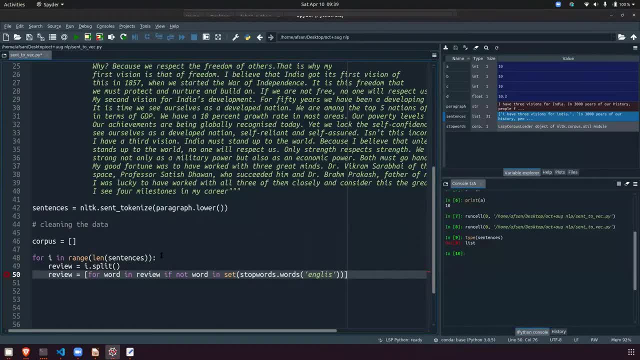 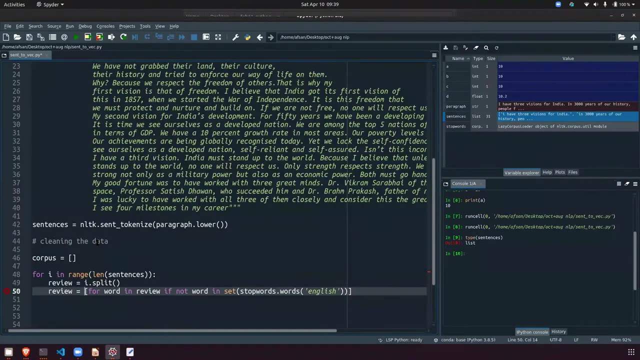 language, so English, so for word in review, if the word is not what is not present in the stock word. so basically I'm just having that work, so okay. so one thing we have missed, and that is instance is initialization. okay, so we have not created any object, okay so 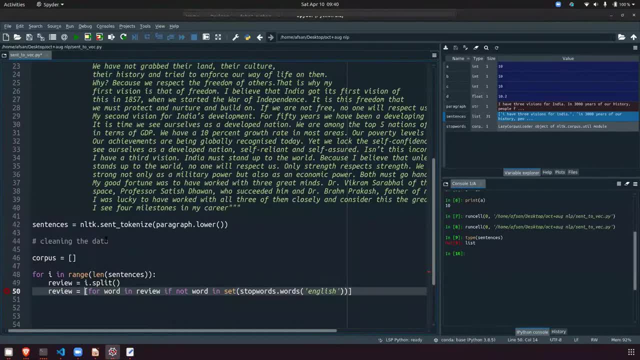 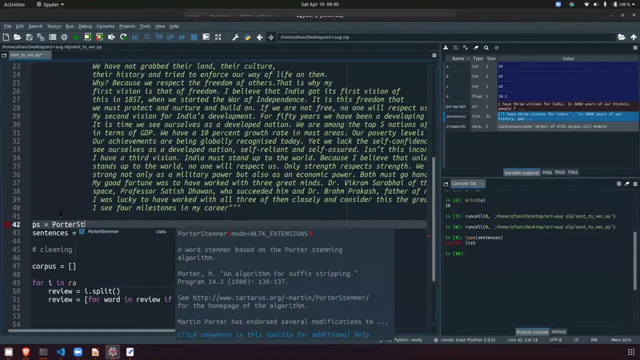 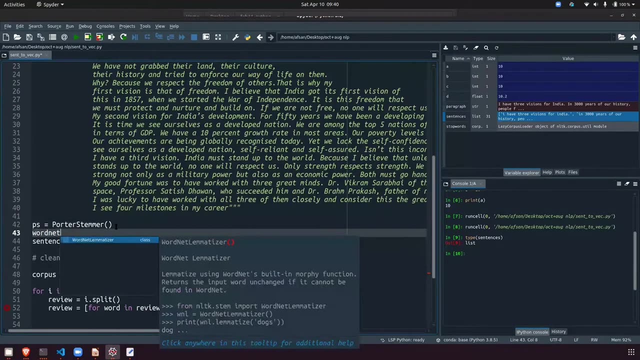 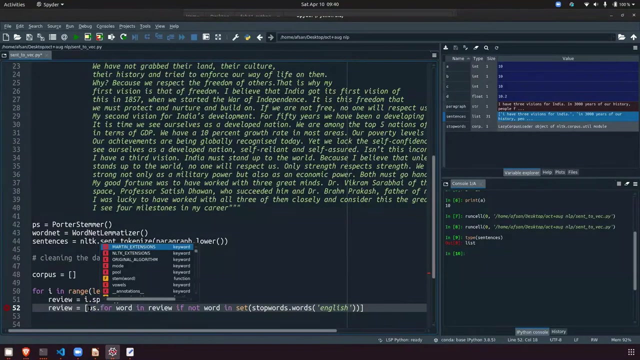 first we have to create the object. that is important thing, right? so what we do is: so we'll do PS equal to quarter stemmer, just call the object, then word net will do word net lemmatizer. that's it, where we just do PS, dot, stem and the word. and after doing this, so what I will? 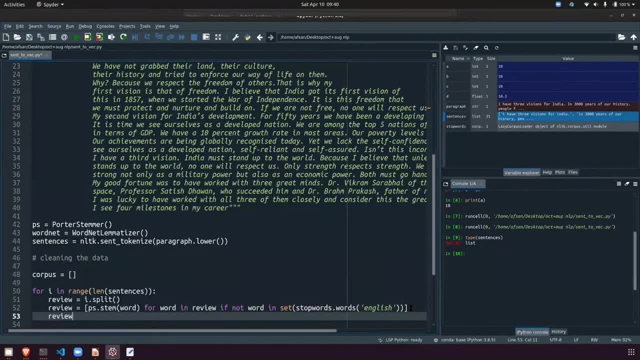 do is: I will just join the sample and mio you would have received will be on a spot moving, move to Champy and then, like you know what, and I will add a class, will now flip to ju slash, j cesa and then create one, then edit path, check with menu, a period or if the server is clicked, option is command. 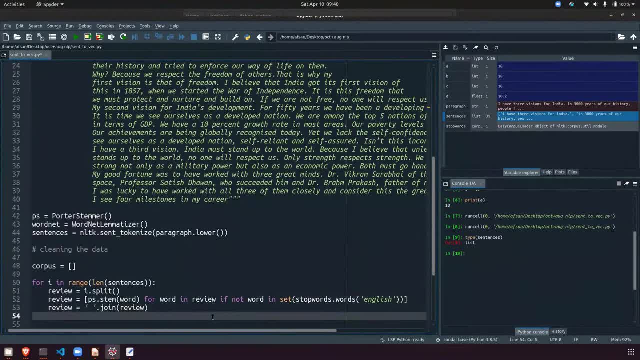 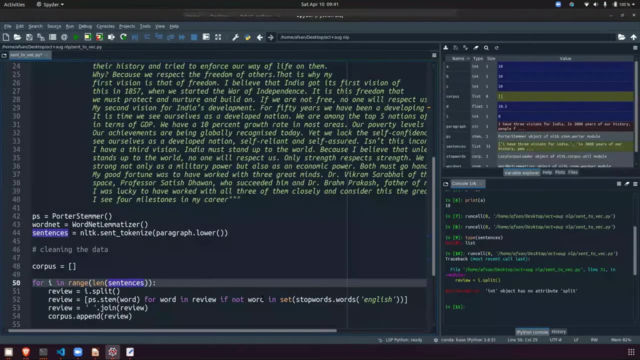 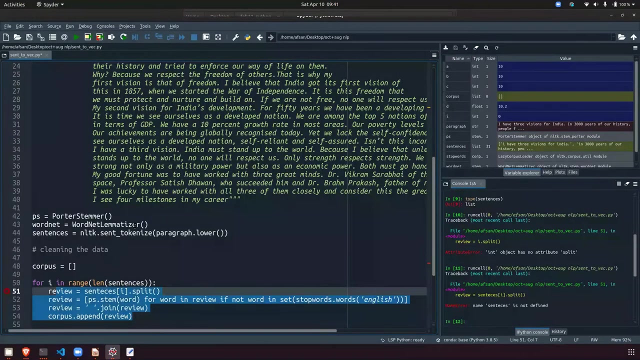 once each particular list value is done with the producing part, I'm again appending it something called as corpus. so corpus dot, append and put it will be. let's try to run this. let's see that what I've done is correct or not. okay, so this will be sentence dot I. so if we file switch it into an, non is missing. so 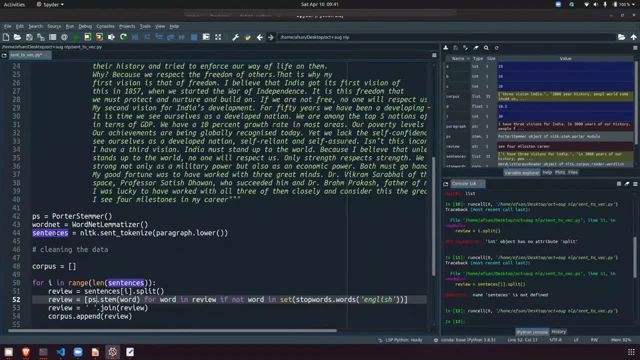 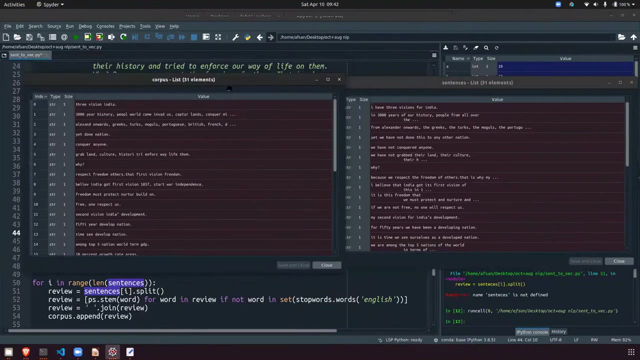 now you can. so there's some falar sentences and they something corpus. okay, special definition between the sentences and the corpus. now, so double click on corpus, open the window, shift towards the left and open sentences and shift towards the right and then. so this was the previous sentence. on the left hand side was the. 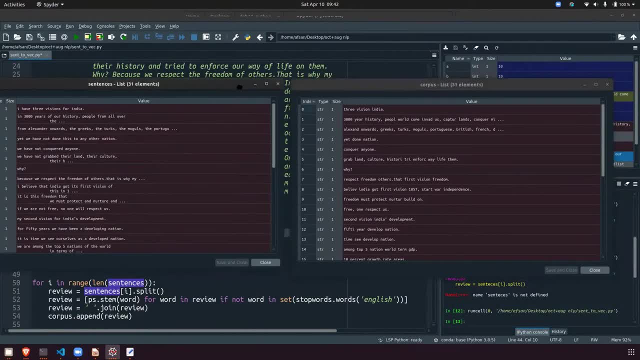 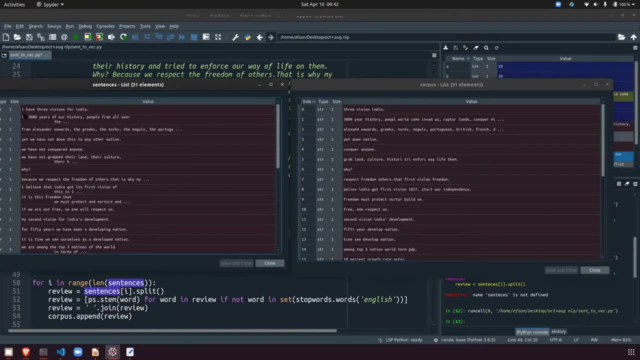 previous okay, or the previous sentence, which you have done. only what sentence organization? and on the right hand side is the clean text. on the right hand has this clean text. look this, for example: I have three visions for India. was the original text. now the clean text is three visions: India in 300 years of our 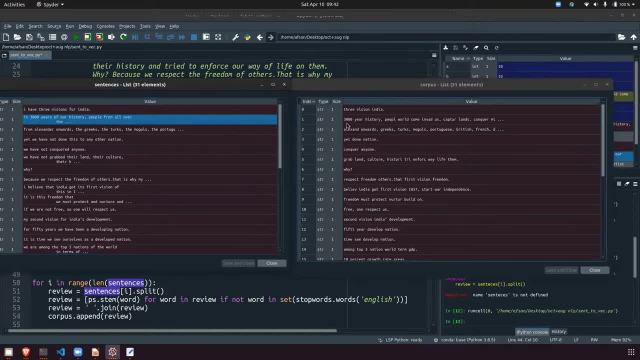 history, people from all over in 300 years history, people, world come invaders and basically it is converting into everything in root form. so stem from, because I am using a infrastemmer, so quote: if you convert everything, then it would be completely free text. it would be completely free text. 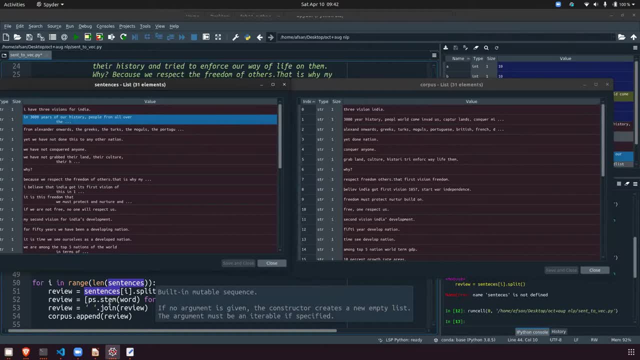 in a stem form so you can use either stem or lamentations. up to you what you want to use. okay, it's up to totally up to you, but the idea is clear to everyone that what we have done till now. so if you want to see the code, just see the code. what i have done. if you have any doubt, just ask me. 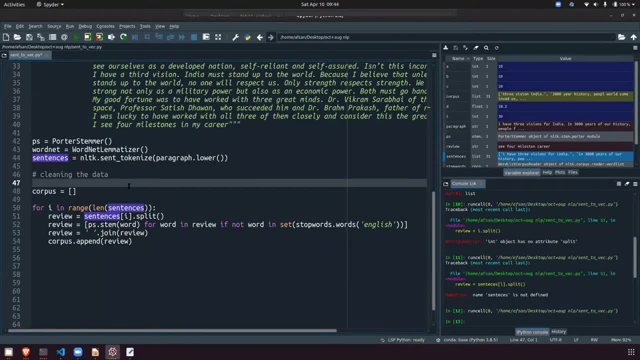 so this what i have done in inside a fall loop, and this following is clear to everyone- but yep, yeah, okay, now what we'll do is we will try to convert this sentence into a vector form. okay, so, in a bag of words, what are the steps that we follow? so the first step is text that we have. 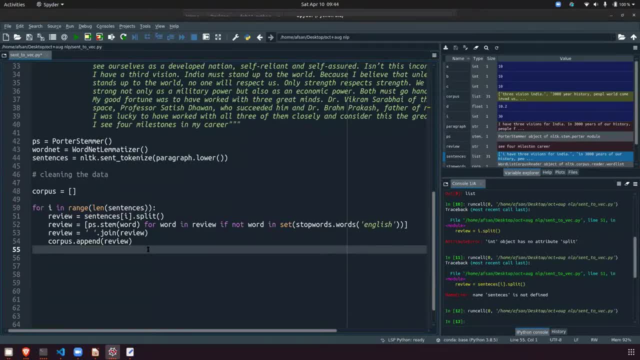 done, then what is next step? make the vocabulary, make a vocabulary, okay, and after the vocabulary, just fill in the table based on the vocabulary. if the word is present, put one. if the word is open, put zero. yes, okay, okay. so what i will do is so, basically, we don't have to do all that step. that is already. 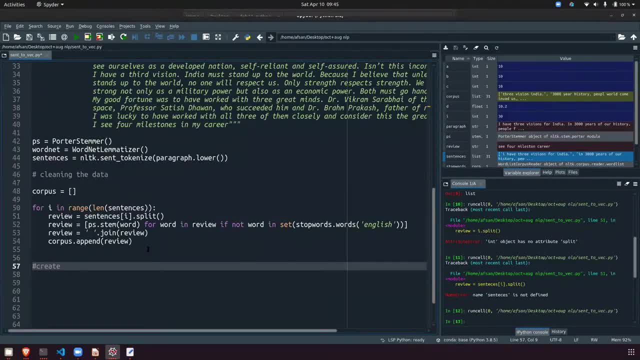 done in a package called as a bag of account vectorizer. so we have to import that package. so, creating a bag of word model, you can say, or you can say bag of word model, layer model, then uh from. so how to import this? okay, so in in nltk, sorry, in sklan. 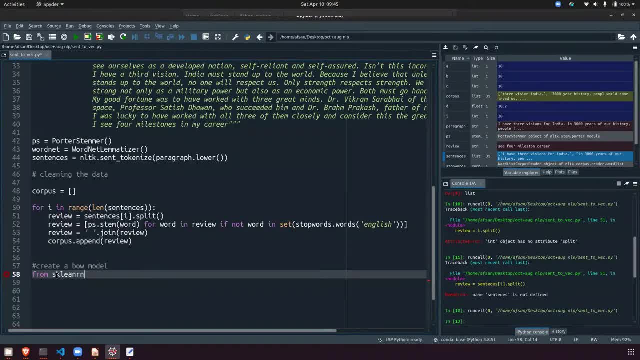 so this is a picture of sklan. okay, in sklan we have something called as feature extraction dot text. okay, so this is the. this is a class, this is the function of the class. okay, and so sklan, feature extraction dot text import count vectorizer. okay, so this, something called as count. 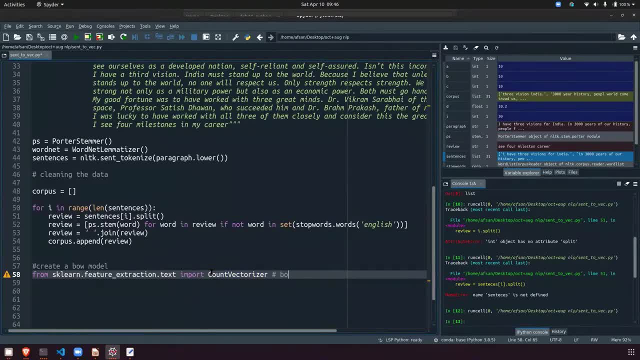 vectorizer. that is equivalent to bag of words. so just change the name, okay, but the function, what it does behind the scene, is that it will be used as a function of the class. okay, so the function, what it does behind the scene, is exactly the same. so how to input back over? so you have to call. 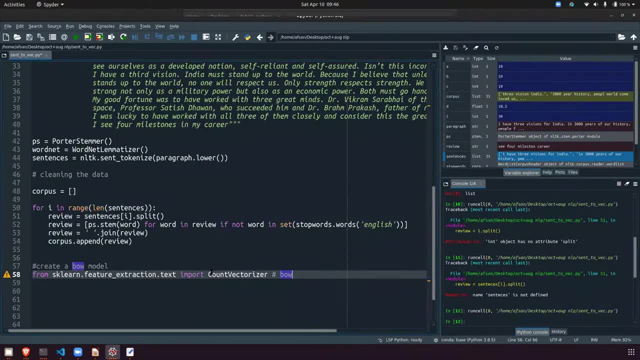 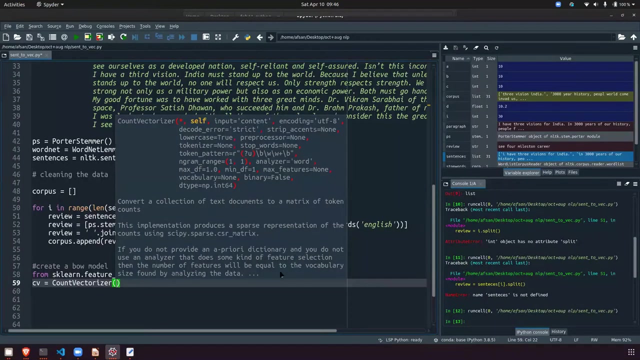 sqln dot feature extraction, dot text import, converterism. so once we have done this. so basically we have to call the object first because it's a class. so count vectorism, c-o-u-n-t vectorizer, and call the class. and the simple thing, what you have to do is just create one variable: x. 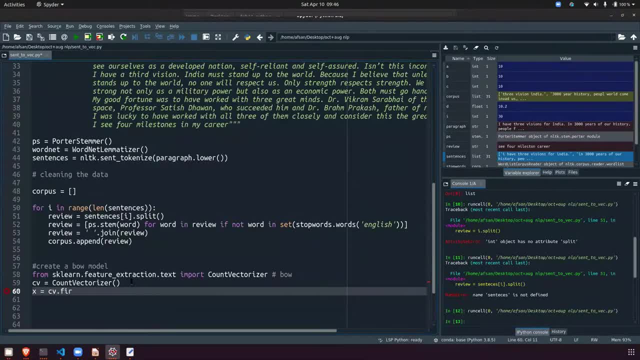 and do cv dot fit transform. that's it. this is the only thing you have to do. so this method you have seen in uh- standard, scalar or normalization, where if you want to convert something into standard or normal way, you do fit. so what is the difference between fit? 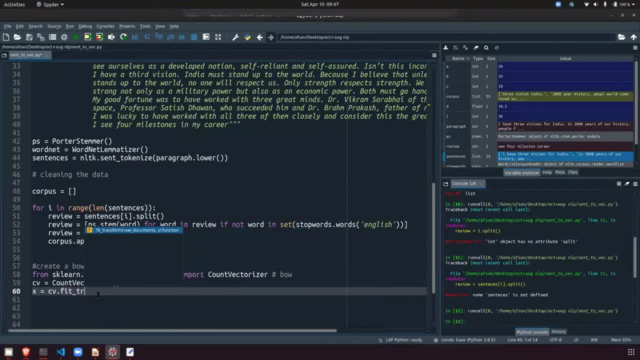 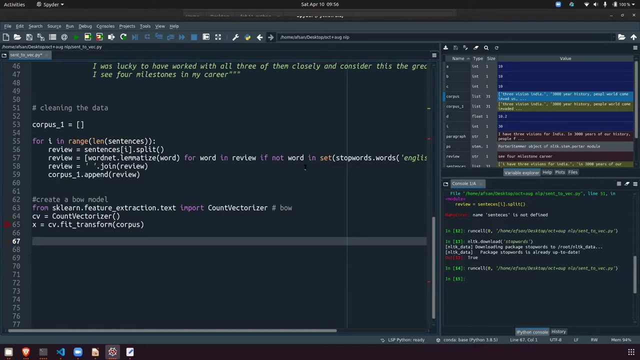 and fit, transform, and you can kind of tell me it just fits to transform this to time. transform okay, 957, okay, like why there is a set of, why there is a it's not set, said just to be on the safe side. if anything is repeating a stopper, just consider the. 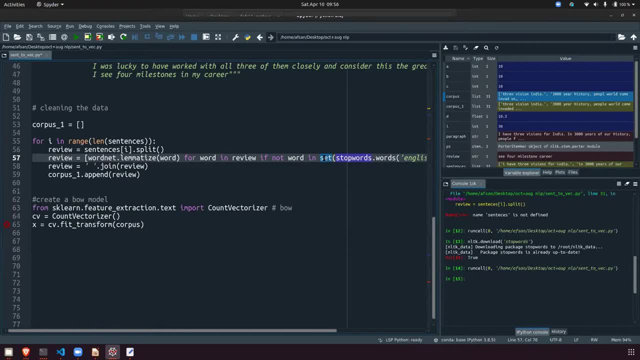 one thing, that's it. so set you can repetition also, repetition is not allowed in set, right, if you remember? so just for that, just be on a safe side. that's it. it's your choice, you want it. okay. can you please share this for loop along in chat. 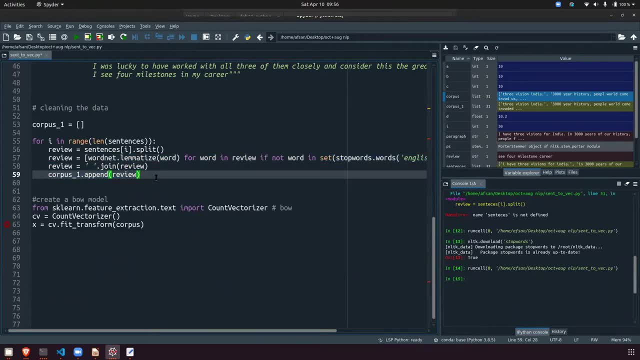 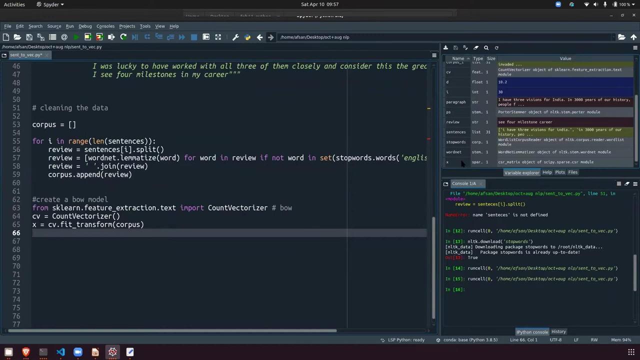 this loop. yeah, okay, finished. so till here, it's good, everyone, what i have done. yes, so i will do the purpose. okay now, if i run this? okay, so i have. so i have got one more variable called as x. okay, now the problem is that this x is this matrix. okay, so, 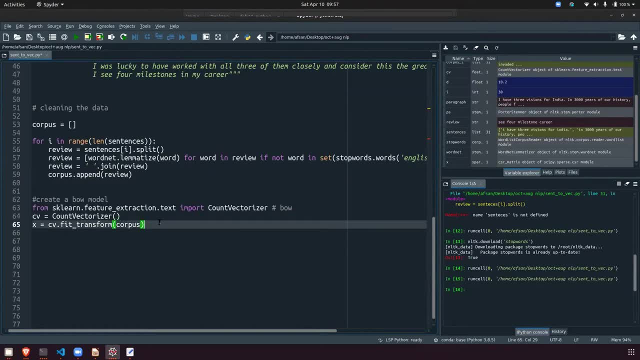 to see this matrix, you have to use something called as two array. okay, so i hope you have learned this. what is two array in pandas or data frame? so two array will convert that everything into array. so two array. so two array will convert that everything into array. so two array. 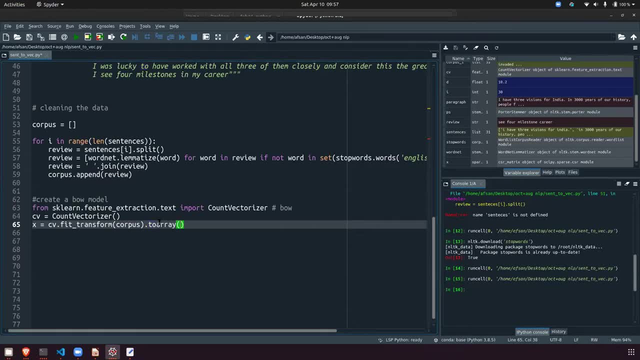 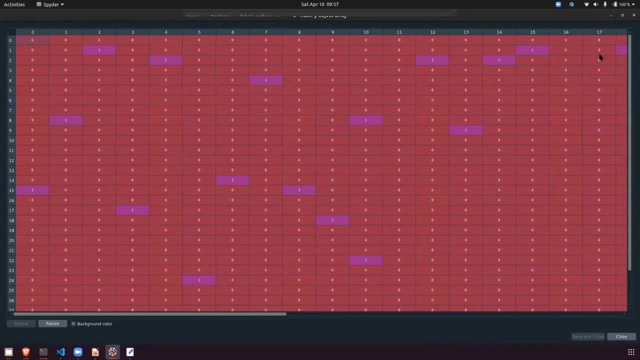 will convert that everything into array. so this is to the x Dinner form. now, when you do this and when you do this and then run this shift tab, and everything is converted into the vector form. so this is what i was saying, this is what i showed you with the help of 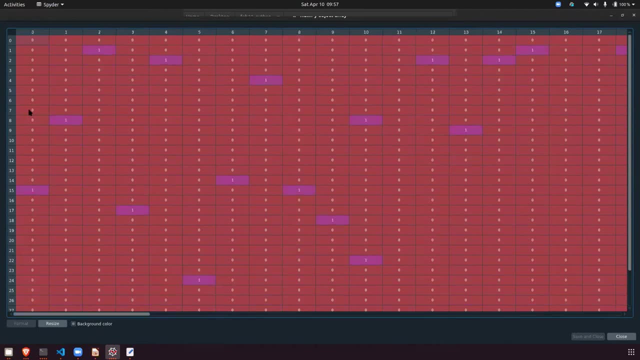 the tables and everything. so this is how it's calculated. so all the values has and this on the top, what is this column? anyone? which one? the column? uh, basically, what is the column in our when you convert all the, each word, each word, okay, is your cabinet that you have? 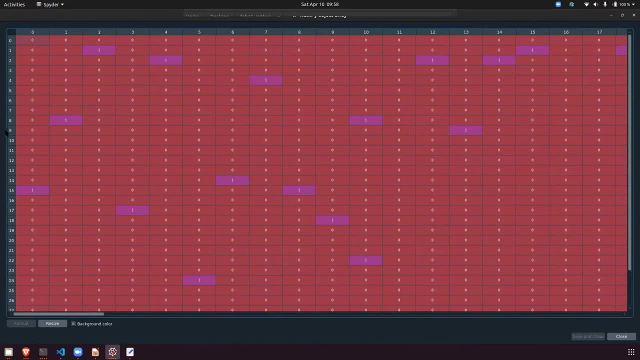 created and on the on the left hand side, it is the sentences. okay, so basically, this is this. everything is a corpus and zero one to the document, if you remember the term. and zero one, two, three, four, five, six, seven, eight, nine, ten- is nothing but uh, uh, features or the vocabulary that you have created. 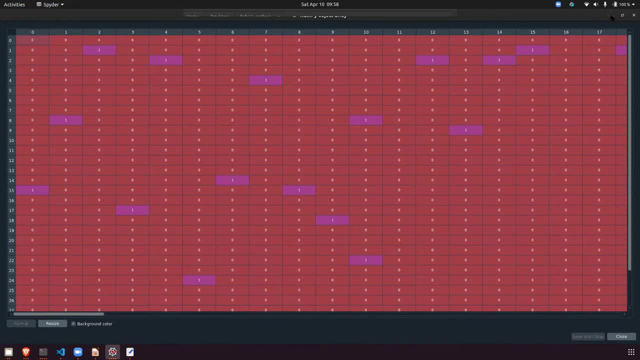 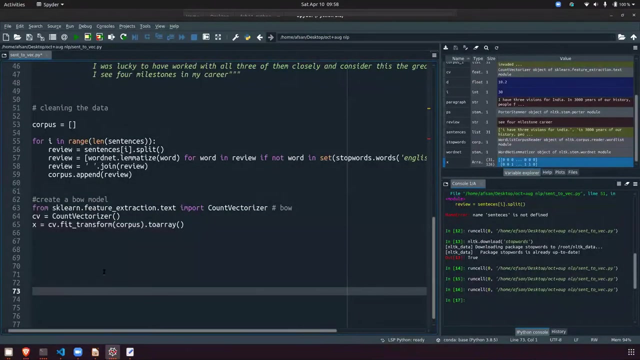 so this is what exactly we have done in the last class, and this is with the practical session. so now, are you able, are you able to relate? uh, can you please show the like uh code for this? yes, yes. so what you have to do is, first, the first step. what you have to do is you have 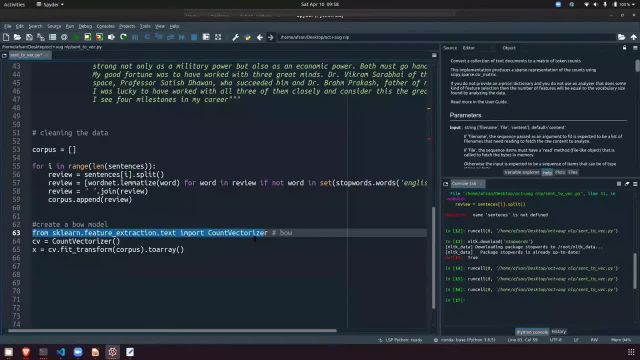 to call the converterizer. so count vectorizer is the name given to bag of words. okay, so don't get confused that i am using something else. no, then you have to call the object of that particular converterizer and then you have to do fit: transform the same thing. 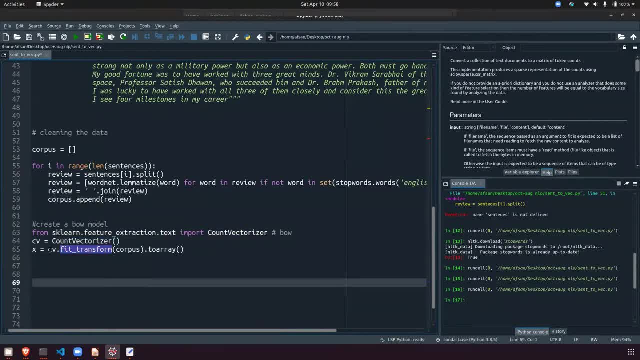 what you have learned in machine learning, the same i am doing here. okay, so cv dot fit, transform corpus dot two array. so behind the scene it will just find the vocabulary and it will try to convert everything in vector form and to arrange to so that we can see the value in our array form. 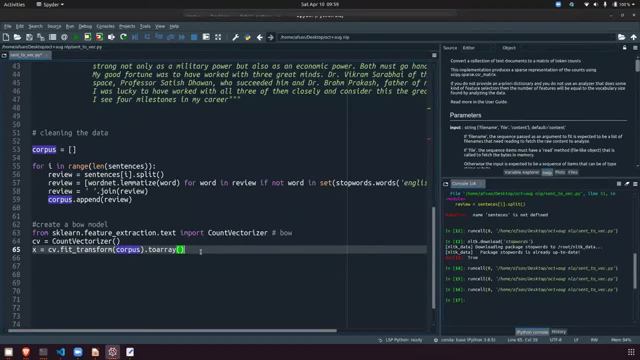 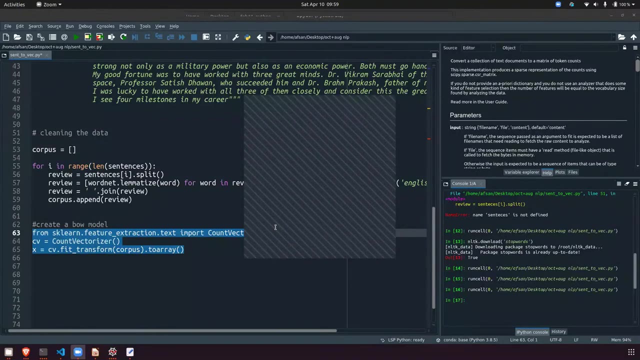 we have done here. okay, got it, thanks. can you just repeat this three last three line: uh, absan, will it still work if i just use fit instead of a transform? it will work, but fit will only try to learn. okay, it will not transform your data into that. that is the difference. 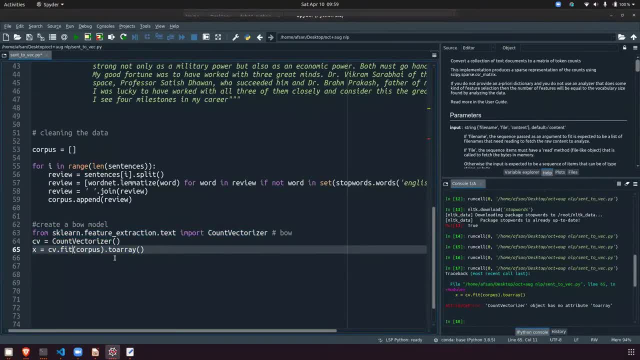 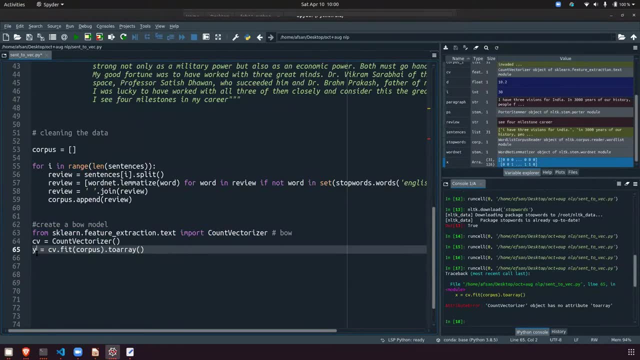 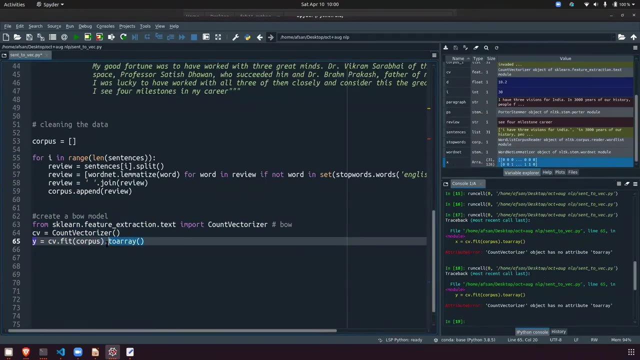 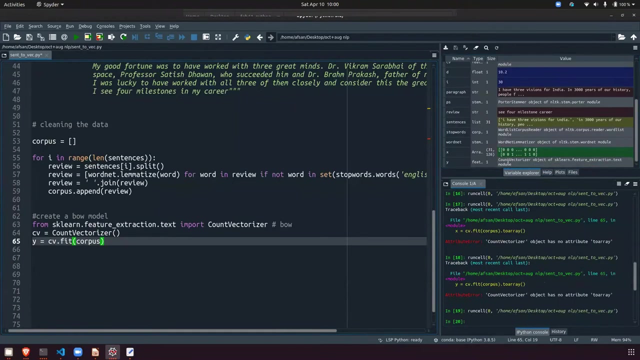 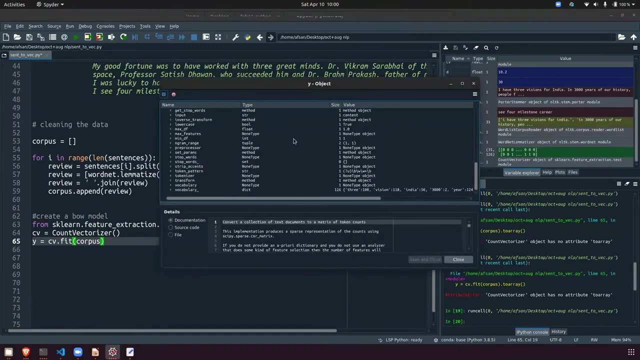 we will do this fit. if you run this, if you go to explorer- okay, this is saved, so i will do x, y, okay, okay, this, so see what fit will do- it will not show you any output. so if you print y, also it will not show any output. 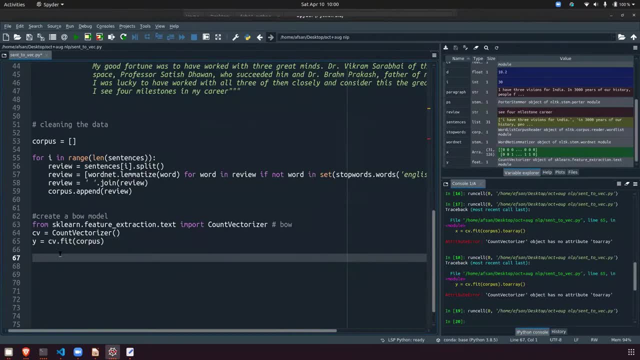 there is a concept of fit and fit transformed in machine that you have learned. so that concept, it will work here. okay, so once you do fit. so what happens on on this corpus? it is learned, it is learning everything, but you have to apply that on corpus also, right? 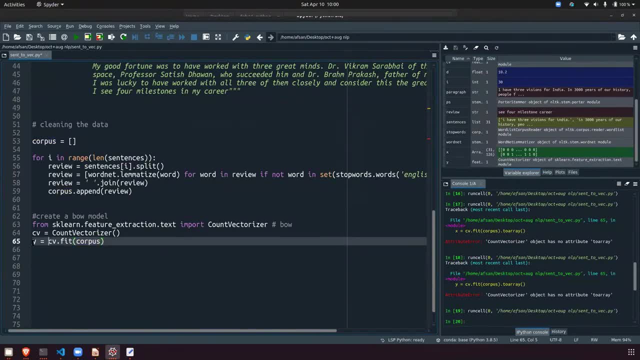 so what you have to do is: so you have done fit. so your y has learned something: that what is the vocabulary and everything. okay now, but it is not applying on corpus because you have not, you have not telling him to apply on corpus, so he's just learning. if you want to apply that on corpus, you 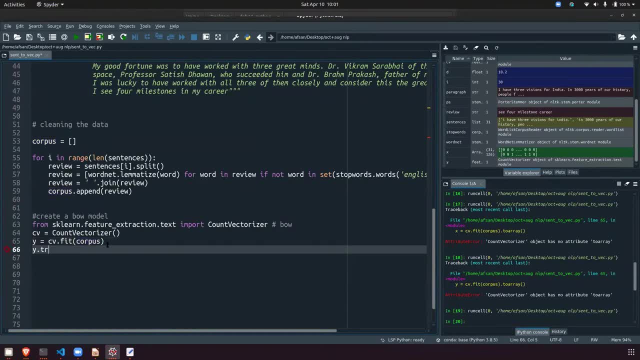 have to do transform, so you can do this way also. so y dot, transform, transform, okay, transform, and just put the corpus that. please transform this corpus for me, based on what you have learned from this field. so, instead of using two, two, two at a time, what you can do is you can do fit and 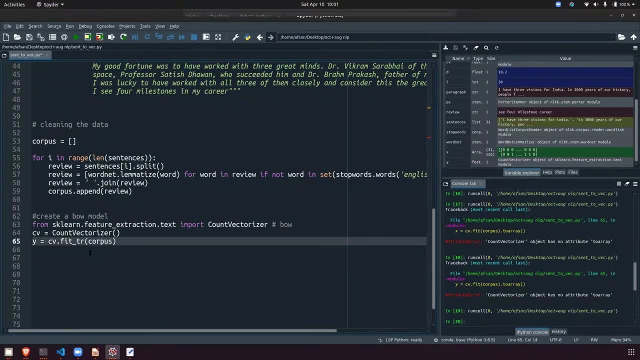 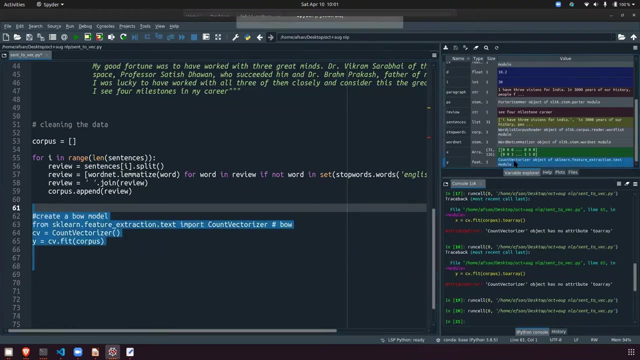 just for transform, so a shortcut. but in this, uh, the output was same. if you know you are not doing the transform right, output is not same. no, so if we remove this, if we remove the transform, and if i run this, see how to not see what is output c. 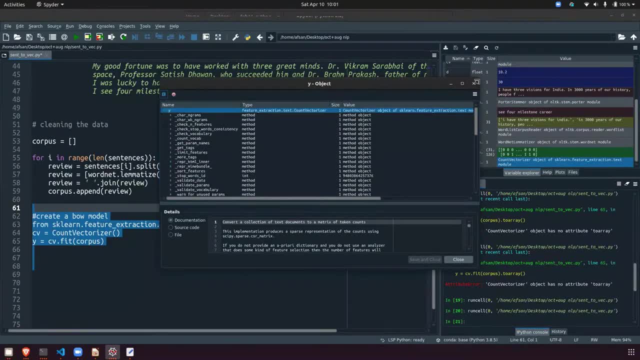 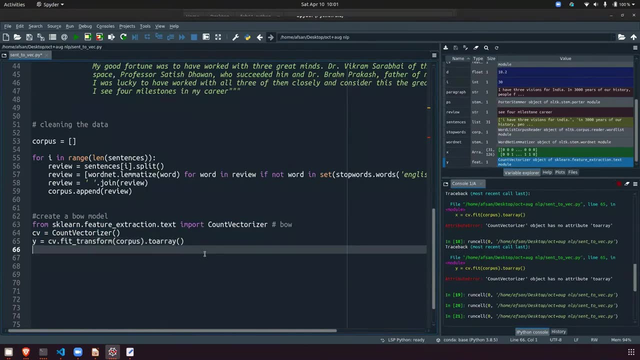 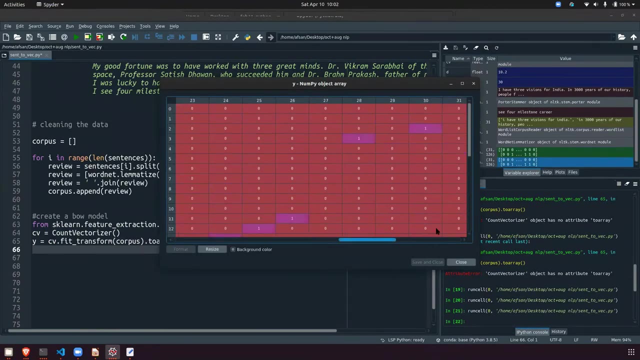 okay, you're getting something else. only now, when you fit transform to array, now the output will be different. so see, now it is converted into proper text, proper, this matrix form or the vector form, so the output is not same. okay, so just just revise this concept of fit transform, okay, so it will be clear. 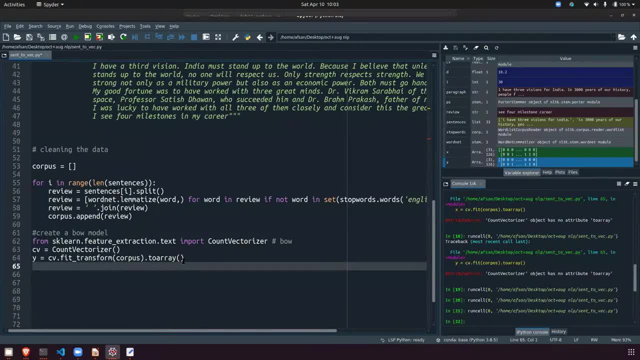 so this uh count vectorizer, or the back over, is given to everyone? yep, okay, and now what is the difference between a bag of words and tf idea? exactly, okay. so basically, in bag of words, if you notice, the answer will be 0 and 1. in tf, idf, it will be between 0 and. 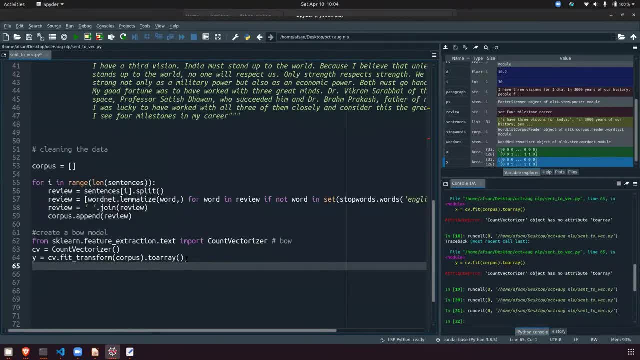 1. this is a difference, okay, so let's try to see that also. so everything will be same, so everything what you have done here will be same. that's the only thing. what i will do is i will just change this particular function. so i will not change this. basically, i will in the down, i will create. 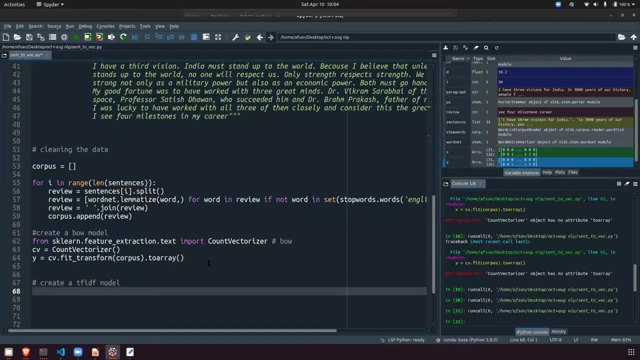 create a tf idf model. so again the same thing. so from sk learn dot feature extraction, dot feature extraction, dot text import. now here we have something called as tf id vectorizer. okay, so the name is maintained here. so tf id vectorizer. and again just uh, so tf equal to just call the objects, just call the class, that's it. tf id of. 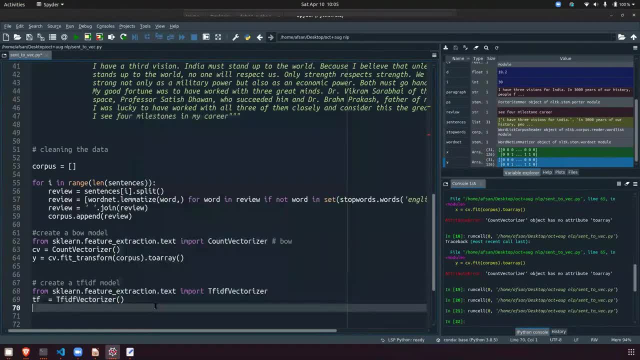 vectorizer and just do fit transform. that's it. this is the only difference you have to do. okay, so fit transform, so copy this, paste this instead of cv, just go tf and just put a variable called as z for this. now, if you try to run this everything, 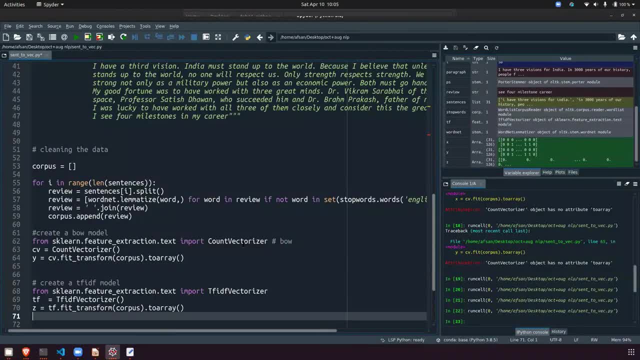 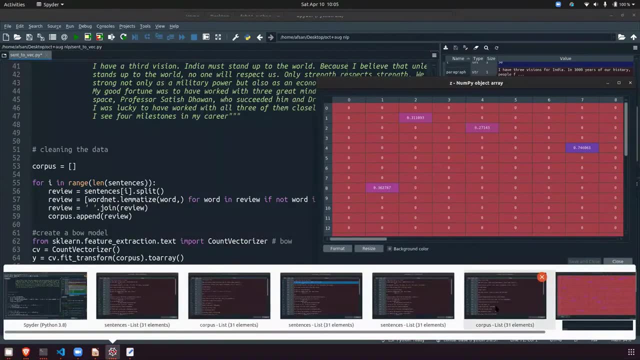 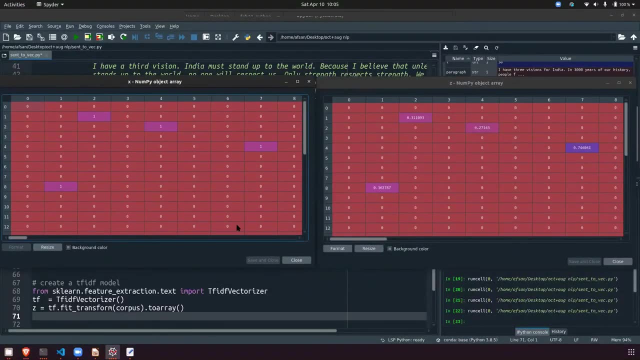 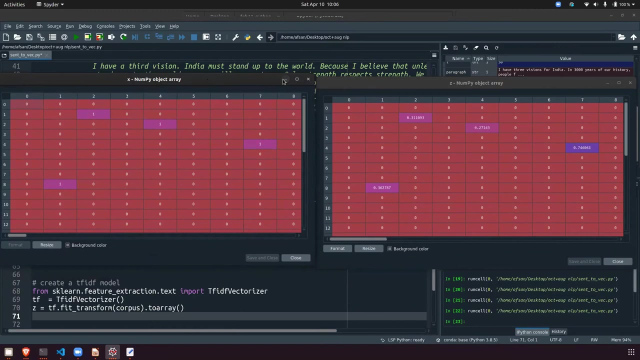 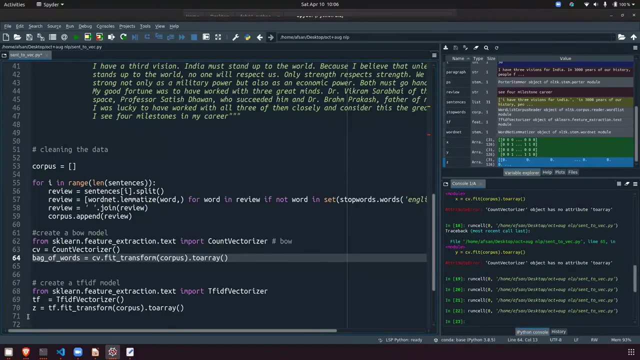 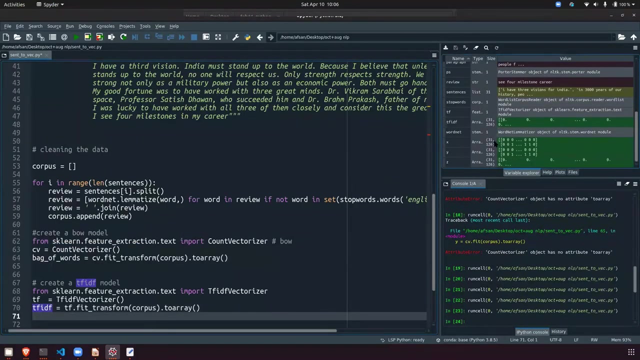 so what i will do is i will open y at one place and z one place. okay, so this is z that is open, and this is x. now, this is a difference between a count vectorizer and a tf idea. okay, you will study yourself. yes, and then 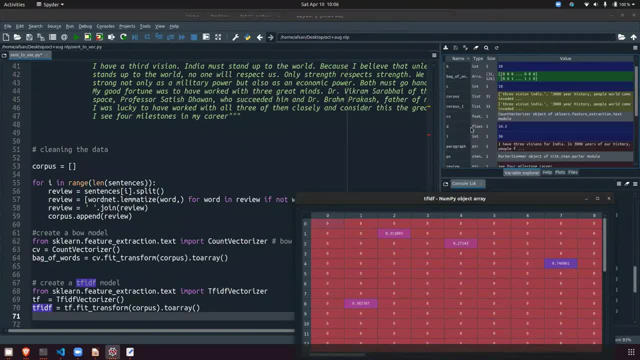 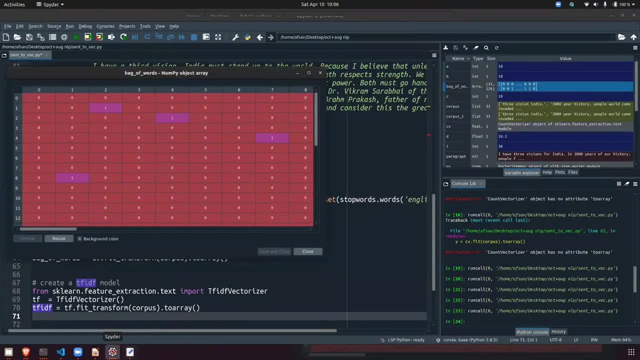 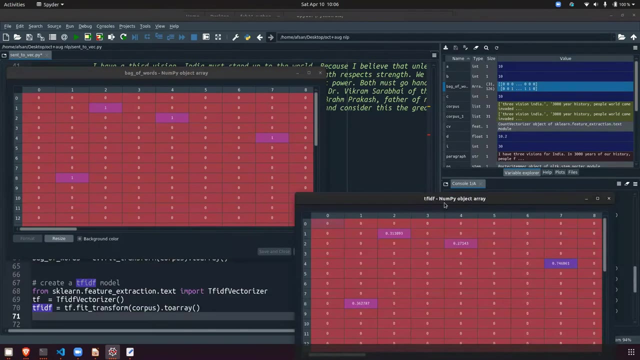 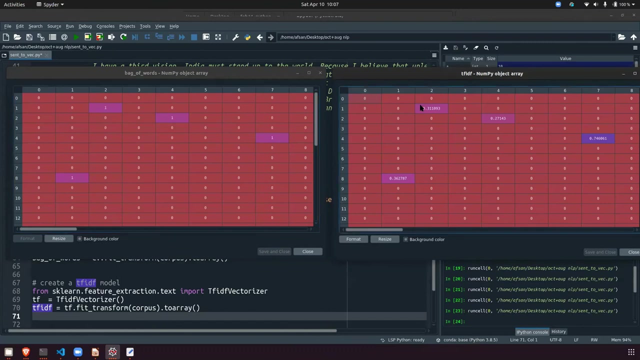 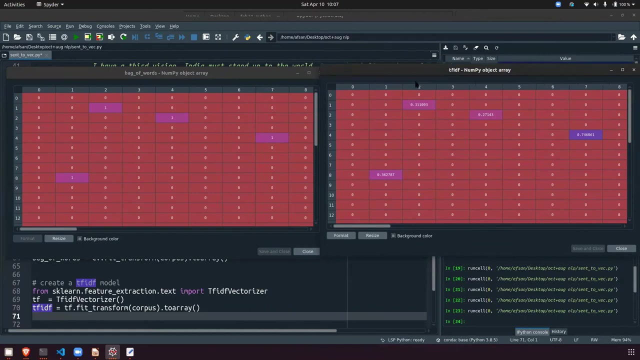 us and you can just play. do So. TF-IDF is more precise TF-IDF. so basically, why you use TF-IDF, suppose? so I have told you in the last class also the importance of TF-IDF is it tries to give the weightage to the important words. 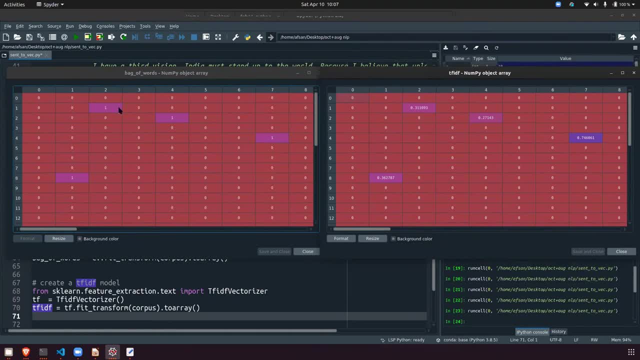 In bag of words, everything is 1, 1,, 1, 1, so my machine learning will understand that, which is an important feature here. right Yeah, But here it is in form of 0 to 1, so my machine learning will understand that 7 features are. 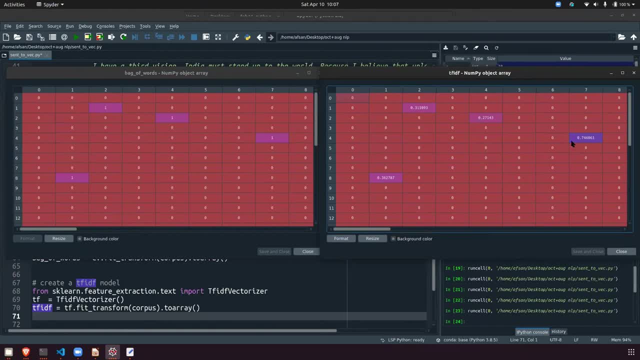 important for this particular row, So it will train on that. so it's like that, okay, So the weightage is given to the each columns. so see, everything is in form of 0s and 0 between 0 and 1, but in this, everything is in form of 0 and 1, so the best method is: 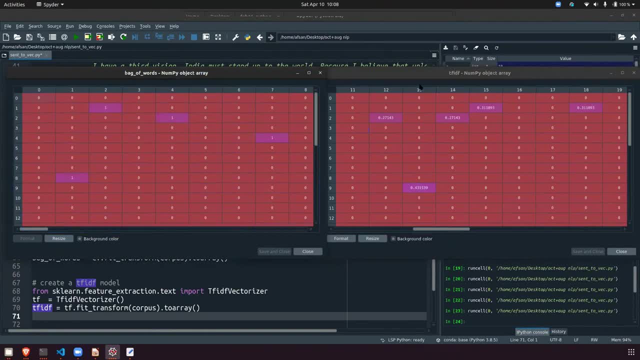 go with TF-IDF. all this, But then the bag of words. I think your machine learning cannot learn from this because there is no weightage, right, Yeah, there is no weightage. there is a weightage, but it is an equal weightage given to all. 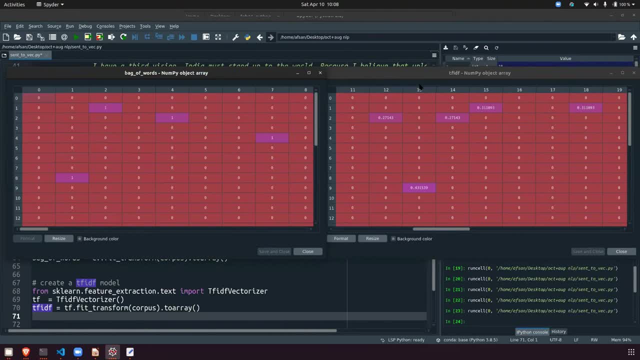 the columns Correct. so then it will be difficult for the model, right? Yeah, it will be difficult. exactly That's why I have given you two examples, So bag of words, So bag of words, and TF-IDF, so that you can relate that which one is better and why. 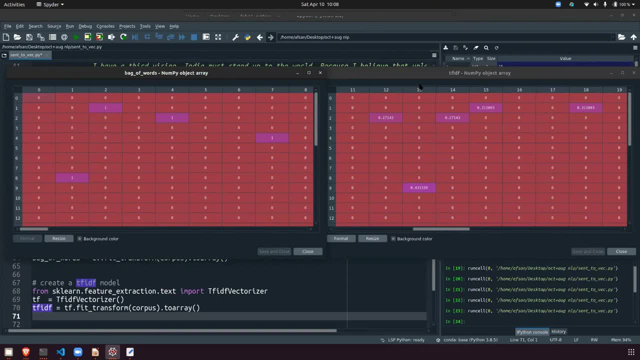 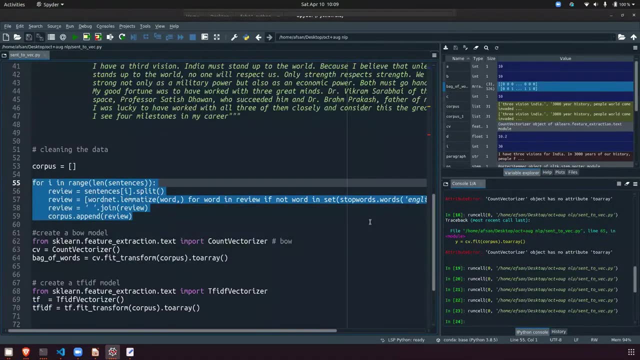 one is better than the other. Now can you relate that? But always TF-IDF is better, right, Yeah, always TF-IDF is better, always, anytime, Okay. So the demonstration of bag of words and TF-IDF is here to everyone.